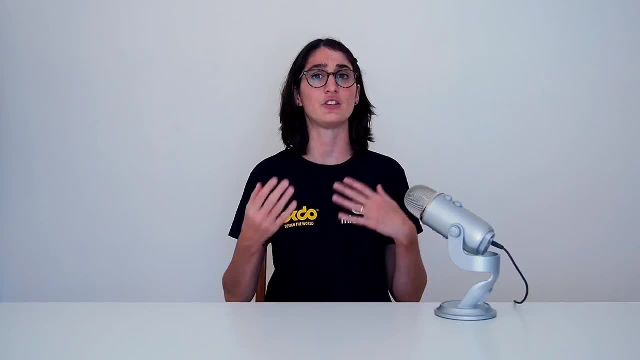 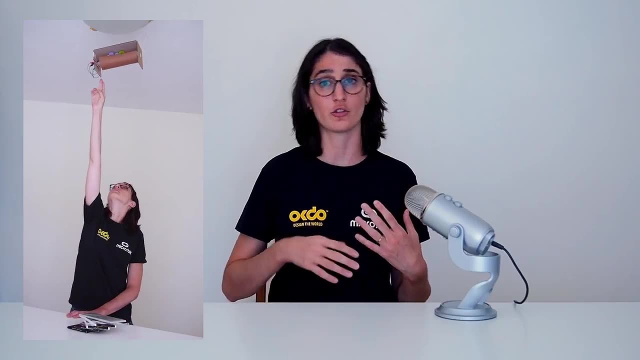 a technical sense and does what it's supposed to. You might have even been doing this as you were building to make sure things work. For my pom-pom booby trap, that means making sure the code works, the motors turn when they're supposed to and the sensor knows when someone touches the chocolate. 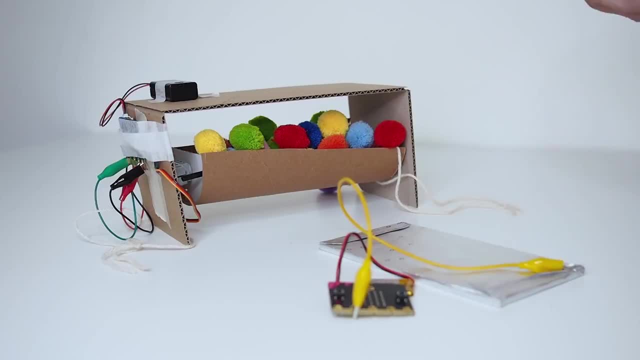 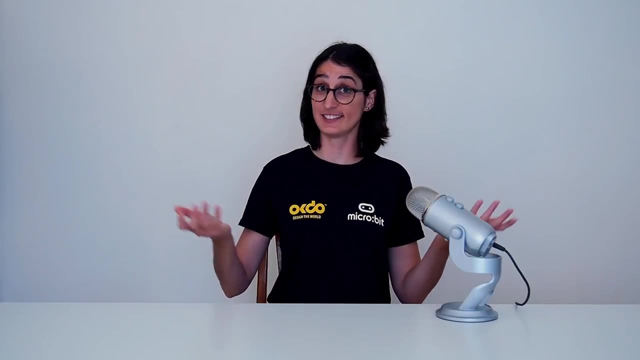 Most of the time the prototype won't work the way you want it to the first time around, but part of testing is figuring out why it doesn't, so you can improve it For this first activity if you haven't already test how your prototype works. 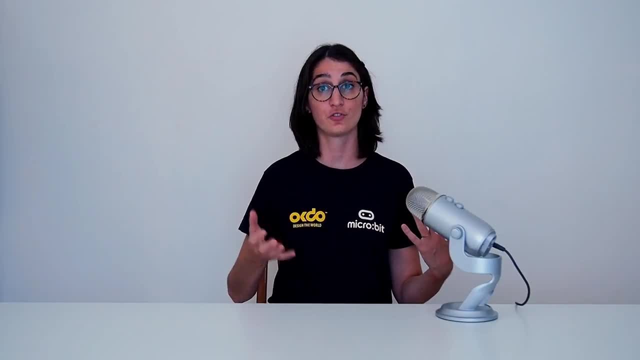 Use your design notebook to take notes on things that don't work or could be improved on, like the motor doesn't turn all the way or the sensor isn't detecting when I touch it. If you think you know why something isn't working, write that down, too. Like 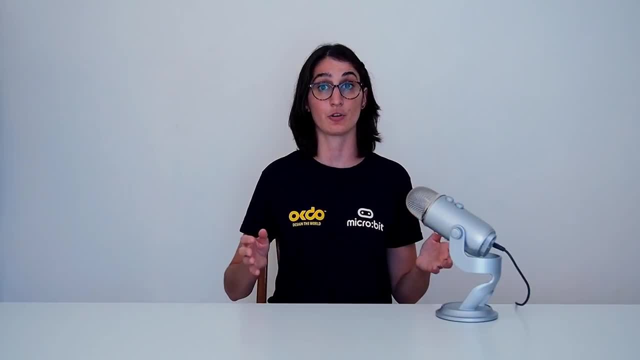 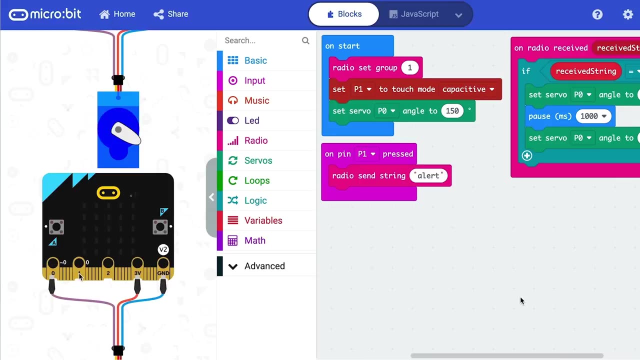 I think I've done it wrong- need to use a different code block. If it's a paper prototype, you may not be able to test it in quite the same way, but you can still do research on the parts you're less sure about, or try coding it with a micro bit simulator. on. 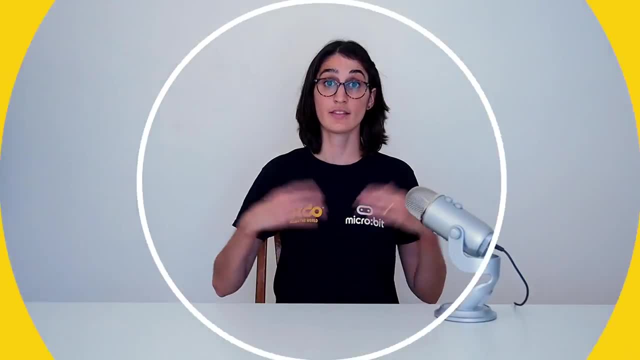 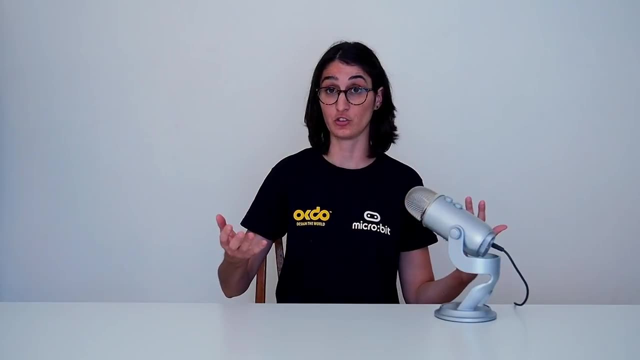 the MakeCode website. The second part of testing is making sure the user wants to use the solution you've designed. This is where I'll do another round of user research, but this time I'll actually have the user test the prototype or show them my paper prototypes. Then I'll do an interview or 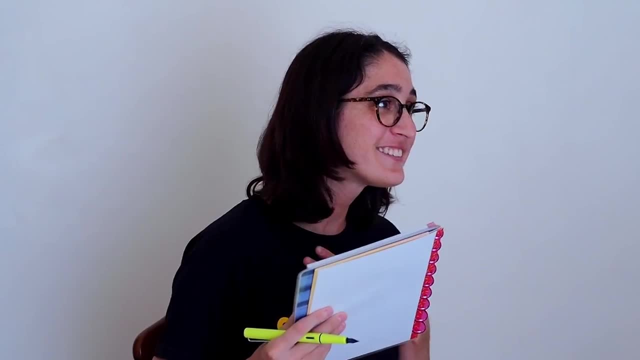 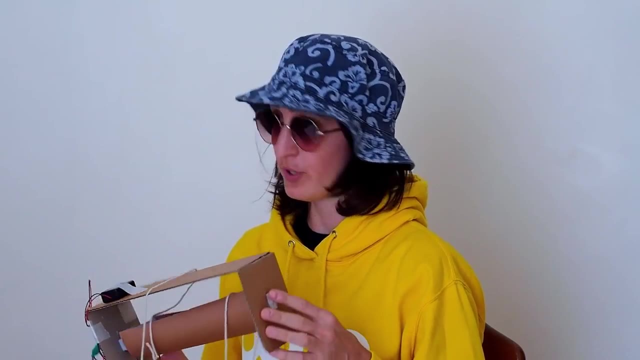 a survey to get their thoughts. Hi, Schmazman, great to see you again. Hi, Jasmine, you too. So, um, what did you think of the prototype I built? Ah, it's pretty cool. Okay, thanks. What specifically did you like about it? Um, I like that it's. 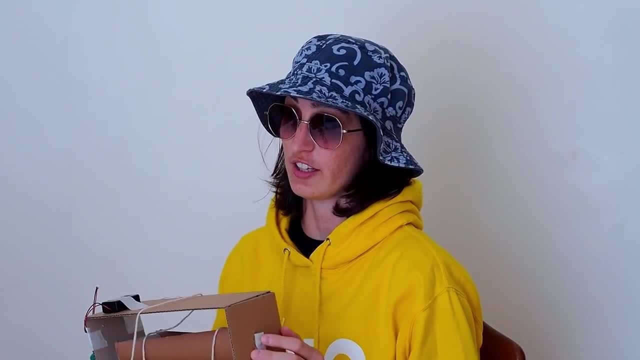 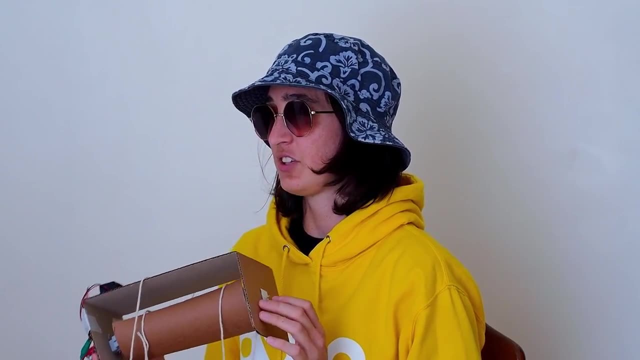 automatic and that the booby trap goes off as soon as anyone touches the chocolate. Thanks. What don't you like about it or think could be better? Mmm, well, I don't like that. I have to clean up all the pom-poms after, Also right now. 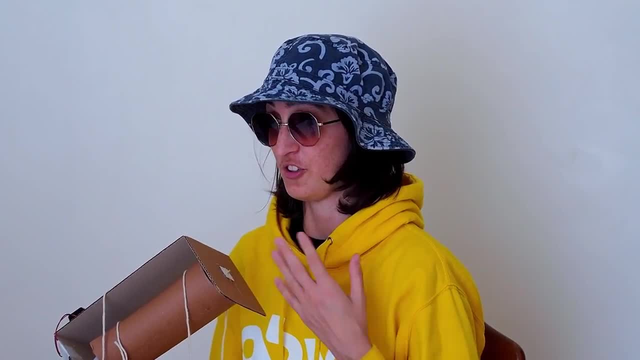 there's no way that I have to clean up all the pom-poms after. Also, right now, there's no way for it to know if the person taking the chocolate is an intruder or if it's just me and I don't want to get pom-pommed. Uh, maybe you could add a. 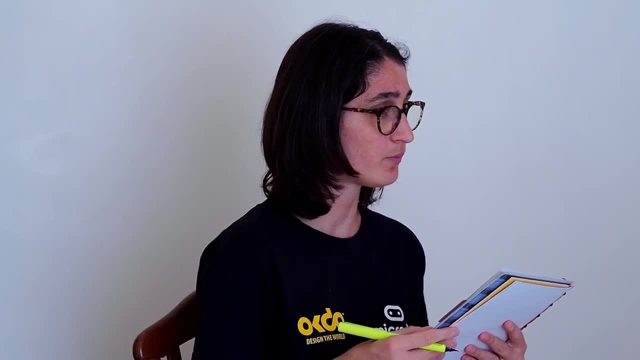 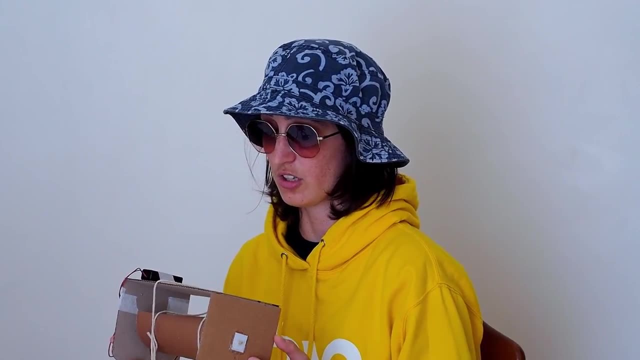 password or something. Great idea, thanks, Um. do you think you would use this at home? Well, to be honest, I think until you fix the issue that it doesn't recognize the real owner of the chocolate, I probably wouldn't. Thanks,